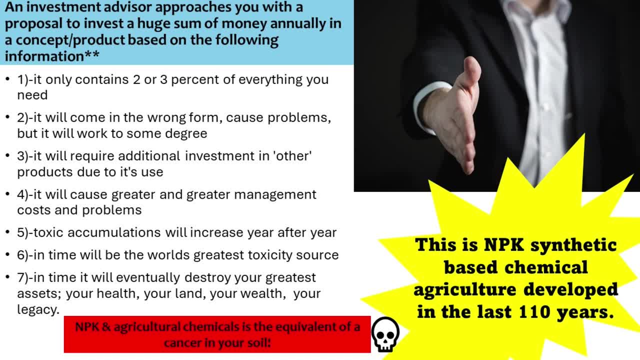 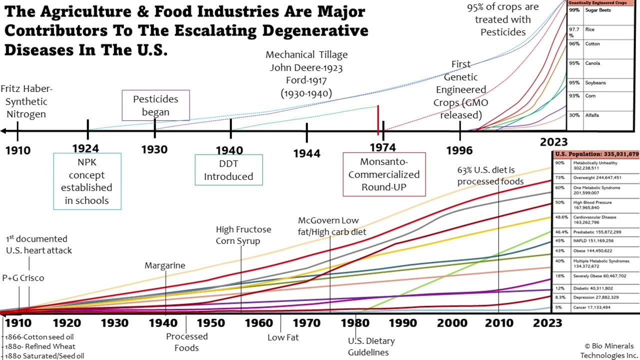 your health, your land, your wealth and your legacy. This is NPK- synthetic-based chemical agriculture that we have developed over the last 110 years. NPK and agricultural chemicals are the equivalent of a cancer in your soil. Let's look at some of the agricultural and food industries. 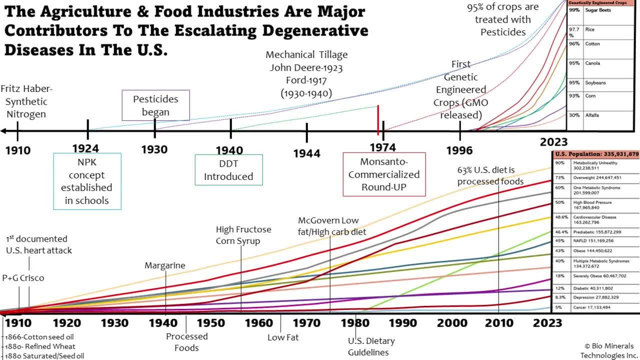 as we move forward, As being major contributors to the escalating degenerative diseases in the US today. 1910 was when we had our first chemical synthetic nitrogen. By 1924, NPK concept had been established in schools. We began using pesticides in 1930.. 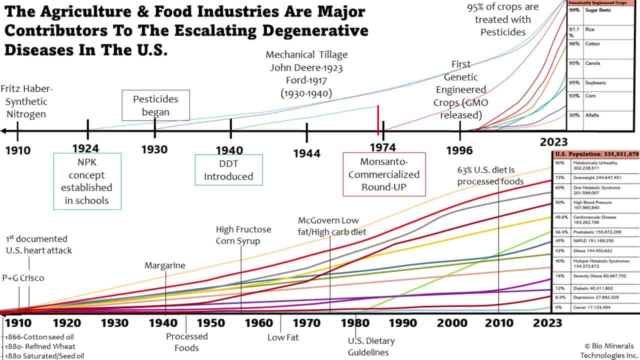 DDT was introduced in 1940. We had progressed with our tillage to where, in the mid 40s, it was very common. DDT was finally restricted in 1972.. Roundup, commercialized by Monsanto, came on the market in 1974. 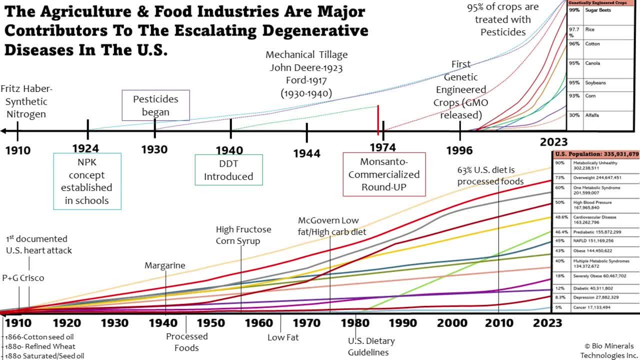 Genetic engineering hit in 1992.. We had a lot of work to do. We started in 1996 and moved forward, And so you look at the rate of genetically engineered crops that exist now in our agricultural systems When we go back and we look at degenerative diseases. 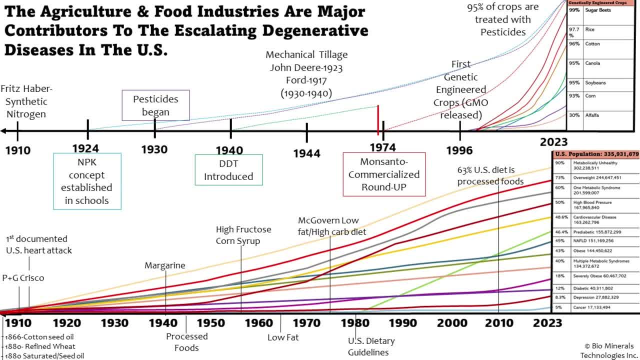 and we look at what changed in our food systems, you will notice that as we switched from from natural saturated fats into seed oils, which began in about 1865, 1866. Then we invented Crisco And then we went from complex and whole food type carbohydrates- 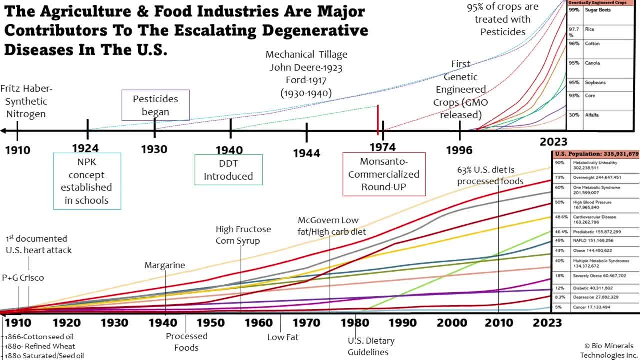 into refined carbohydrates, And we began to replace our natural saturated fats with seed oils. We replaced our whole foods with processed foods, And so we had our first documented heart attack in the United States in 1912.. We began introducing margarine instead of butter and lard. 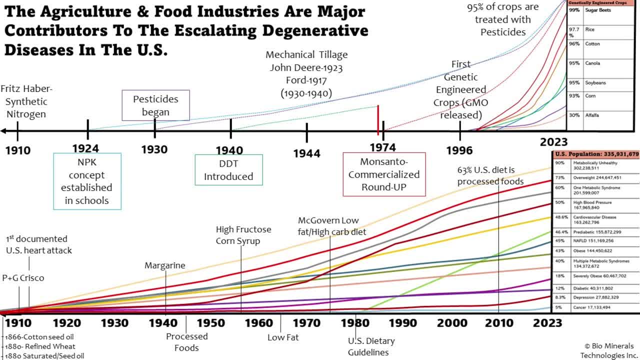 Our food processing began in the mid 1940s. High fructose corn syrup came in about 1957. And then we went to the United States. There was a big push in the 60s and 70s to go to a low fat diet. 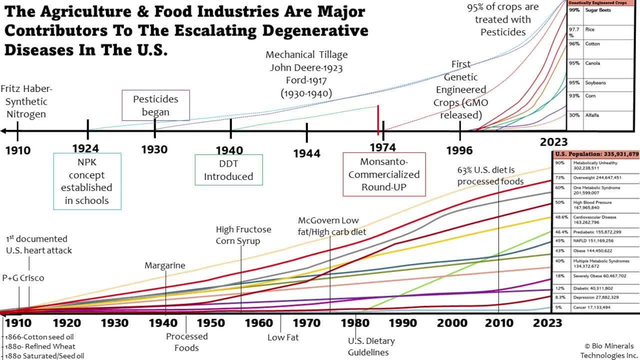 And any type of natural saturated fat was demonized. McGovern went through on regulatory things to put food into the school lunch programs. The US dietary guidelines came out which were to go into seed oils, vegetable oils, processed type oils instead of saturated fats. 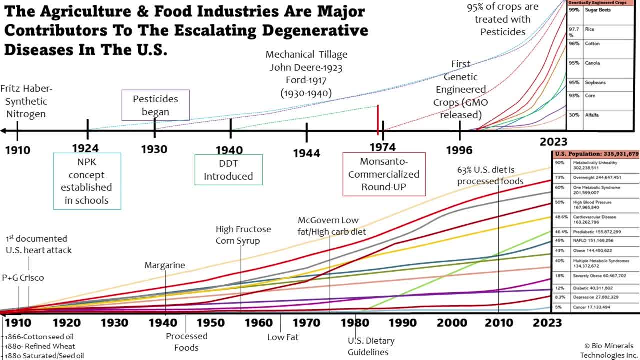 Those were all demonized, The cholesterol boogeyman came out of the closet By 2010,. 63% of the US diet was processed food, which is heavily, heavily influenced by refined carbohydrates and vegetable oils. And you know. 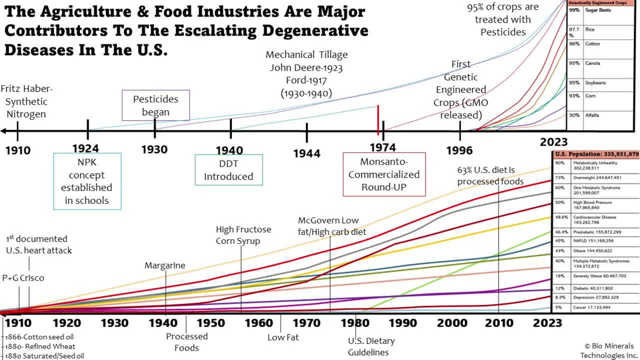 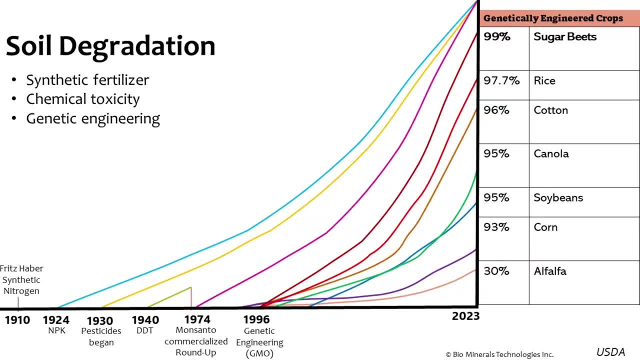 that was a big push And you know you look at the degenerative diseases that have come from this: Our soil degradation, synthetic fertilizers, chemical toxicity and genetic engineering. So this is when we began to implement these agricultural changes and practices. 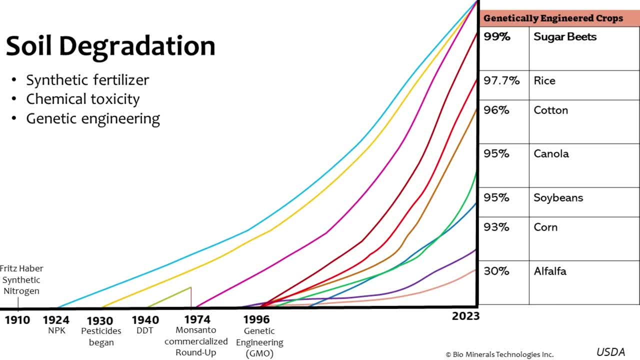 We went from a natural biological system into a synthetic fertilizer, heavily supported by chemical toxicity and genetic engineering. 99% of our sugar beets are genetically engineered, 98% of our rice, 96% of our cotton, 95% of canola we produce. 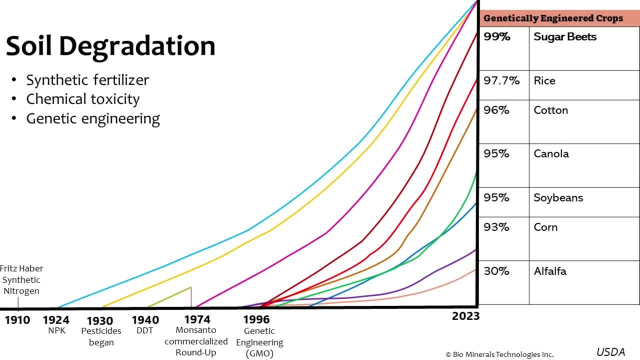 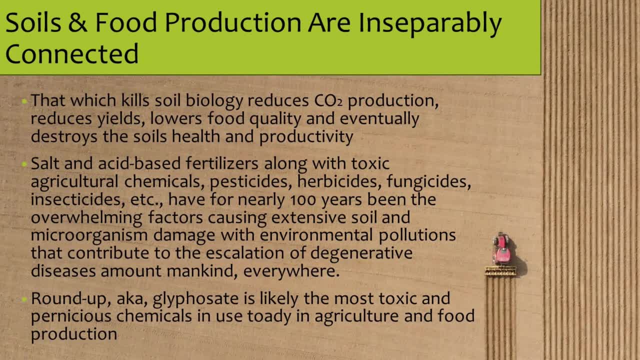 is genetically engineered: 95% of the soybeans, 93% of the corn and up to 30% of the alfalfa. Soil and food production are inseparably connected. That which kills soil biology reduces CO2 production. It reduces yields. 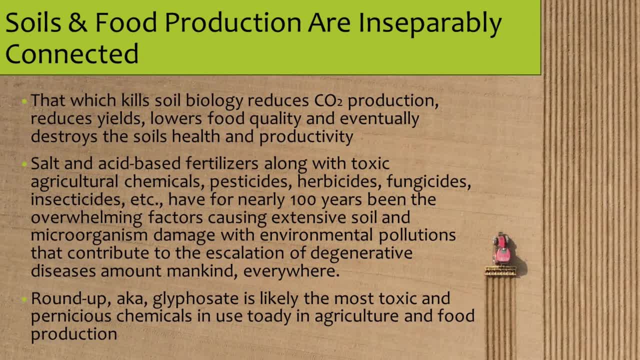 it lowers food quality and eventually destroys the soil's health and its productivity. Salt and acid based fertilizers, along with toxic agricultural chemicals like pesticides, herbicides, fungicides, etc. have for nearly 100 years been the overwhelming factors causing extensive soil. 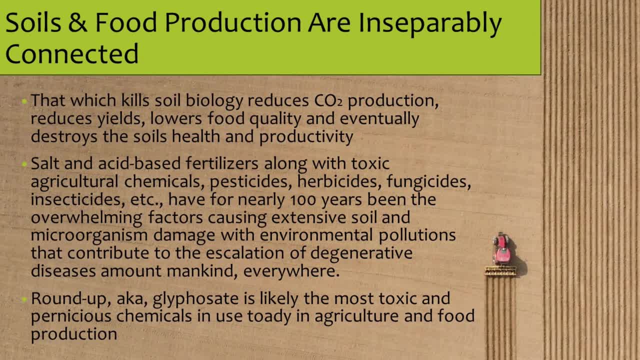 and microorganism damage With the environment, pollutions that contribute to the escalation of degenerative diseases among mankind everywhere. Roundup glyphosate is likely the most toxic and pernicious chemical in use today in agricultural and food production. There are three patents. 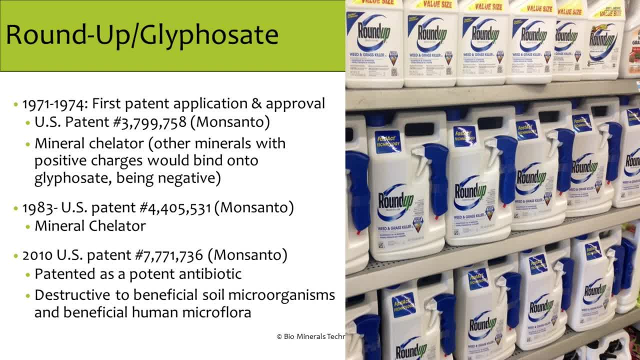 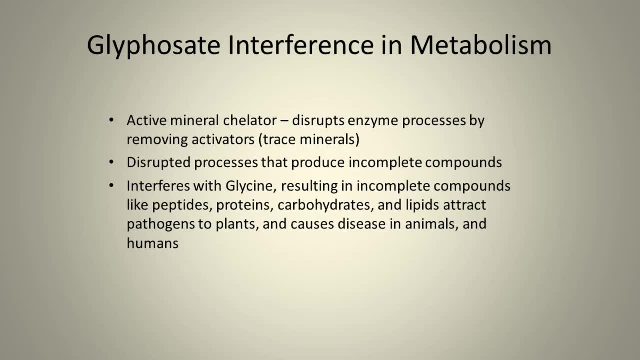 on Roundup, Two of them as mineral chelators and the latest, in 2010, as a potent antibiotic. This is very destructive to beneficial soil microorganisms and beneficial human microflora. Glyphosate interferes with metabolism. Active mineral chelator. 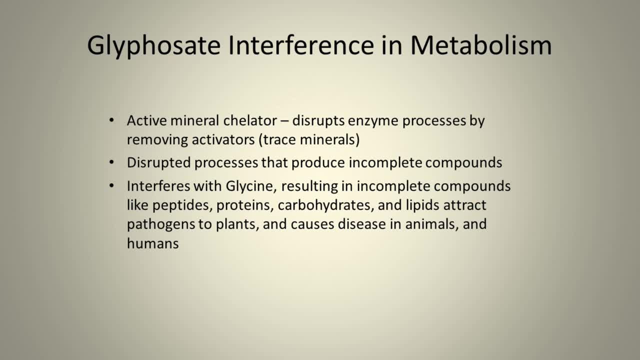 disrupts the enzyme processes by removing the activators. Glyphosate is negatively charged. Trace elements are typically positively charged, so they bind to each other and this removes the trace element from activating enzymes. It disrupts the processes and produces incomplete compounds When these enzymes 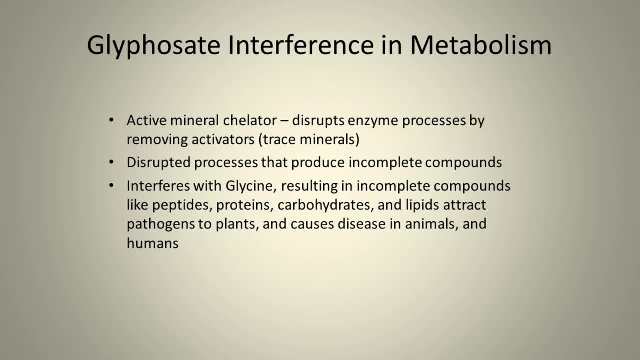 cannot fully function. they do not produce complete compounds. It interferes with glycine, resulting in incomplete compounds like peptides, proteins and lipids or fats. This attracts pathogens to the plant, causing disease in animal and mankind. Glyphosate kills lactobacillus. 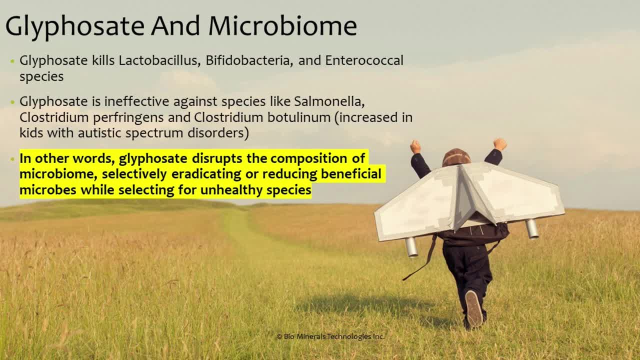 bifidobacteria and enterococcal species. Glyphosate is ineffective against species like Salmonella, Clostridium perfringens and Clostridium botulinum. Clostridium botulinum is found increased in. 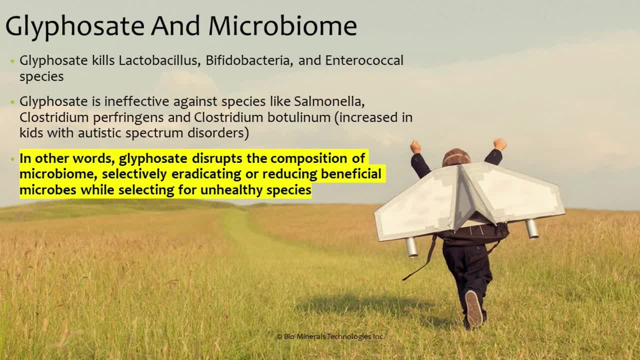 kids with autistic spectrum disorders. In other words, glyphosate disrupts the composition of our microbiome by selectively eradicating or reducing beneficial microbes while selecting for unhealthy species. It does this in our gut. It does exactly the same thing in the soil. 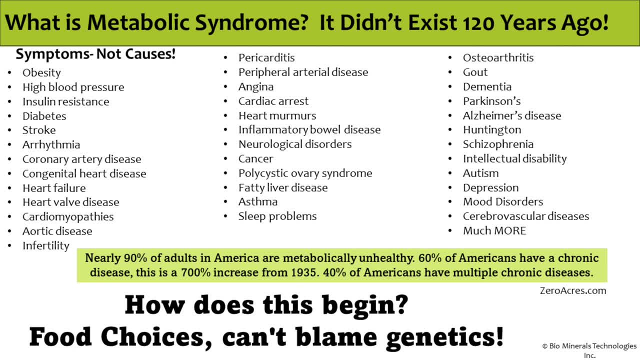 So what are we talking about with metabolic disease? These didn't exist 120 years ago. So you start looking down the list. there is a massive, massive increase in these metabolic diseases that have come from our agricultural and our food system changes, Basically going from natural. 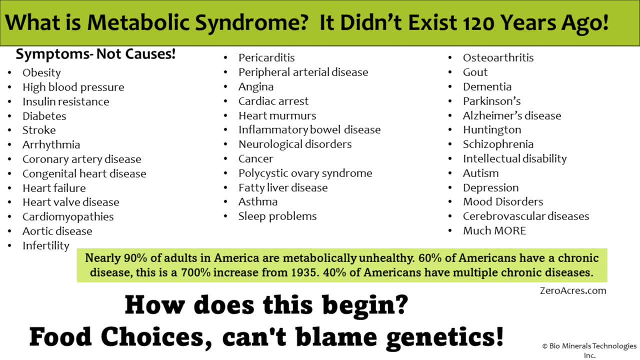 systems that are biological based into chemical systems that are fertilizer based. Nearly 90% of adults in America are metabolically unhealthy. Actually, it's over 90%, It's 93.4 or 93.6%. You can find 5 to 6. 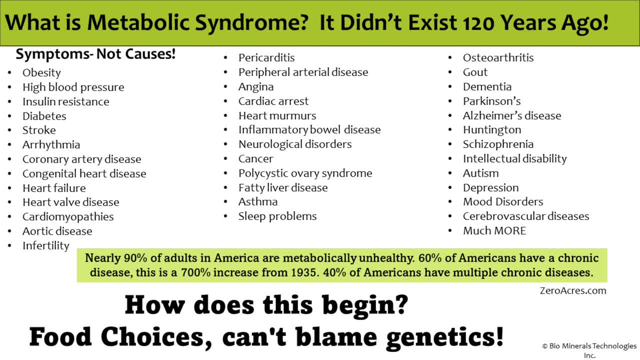 out of 100 people that are metabolically healthy. today, 60% of Americans have at least 1 chronic disease. This is a 700% increase since 1935.. 40% of Americans have multiple chronic diseases. The human disease timeline. 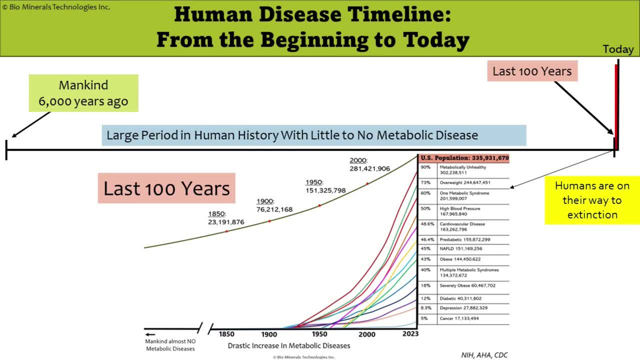 When you go back on human history, there has been very little to no metabolic disease. In a biblical sense you go back almost 6,000 years And we don't have a history of these kind of diseases. But in the last 100 years 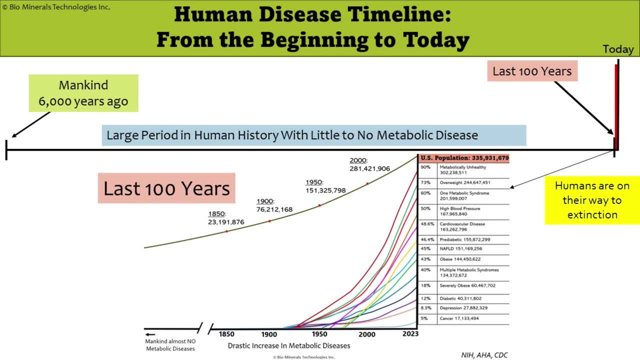 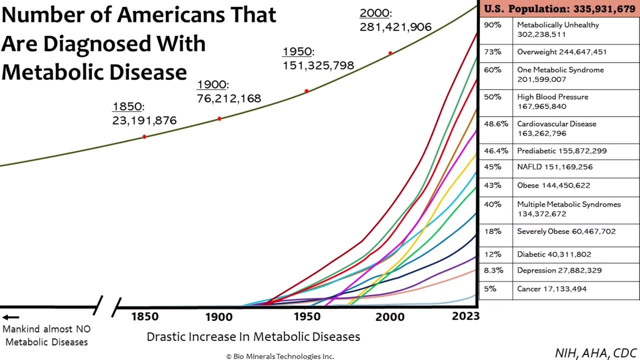 we have escalated the disease in the human population to these types of unimaginable levels. At the rate we are going, this is a path to extinction. The US population. we can go back and we can start looking at the changes in our agricultural systems and in our food systems. 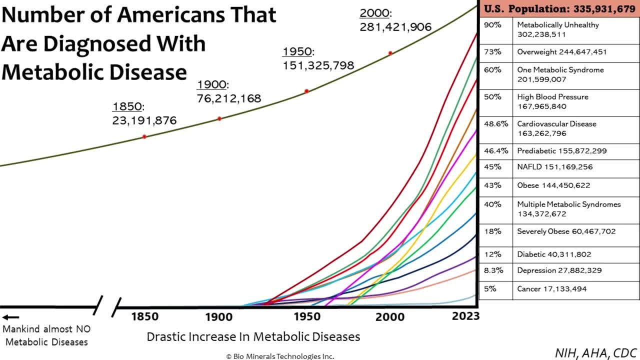 And you can track how metabolically unhealthy we are. We have approximately 336 million people in America. Over 300 are metabolically unhealthy- 73% of our population. 244 million are overweight. At least 200 million have 1 metabolic syndrome. 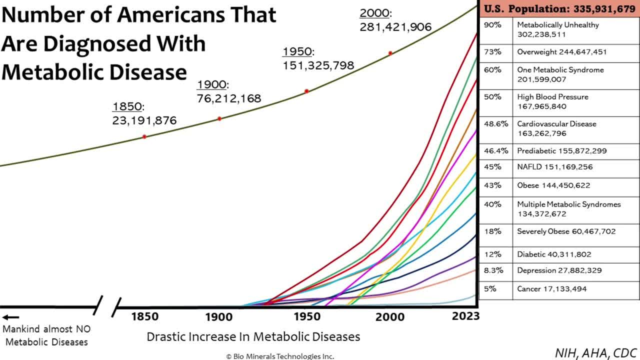 50% of our population. almost 168 million people have high blood pressure. Almost the same amount have cardiovascular disease Pre-diabetes in America at 46.4% or 156 million people. 45% of our population non-alcoholic. 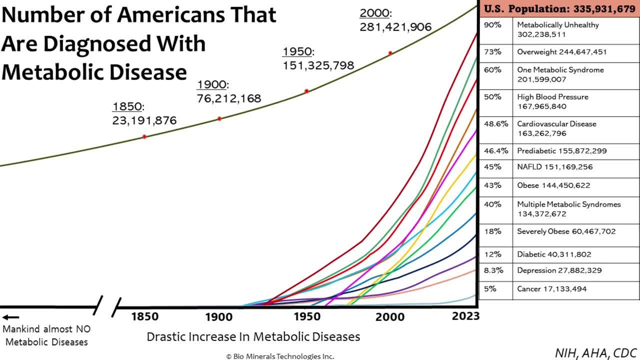 fatty liver disease: Over 150 million people. 43% of our population is obese. That's 144 million people. 40% of our population has multiple metabolic syndromes: Another 100 or 135 million people- 18% of the population. 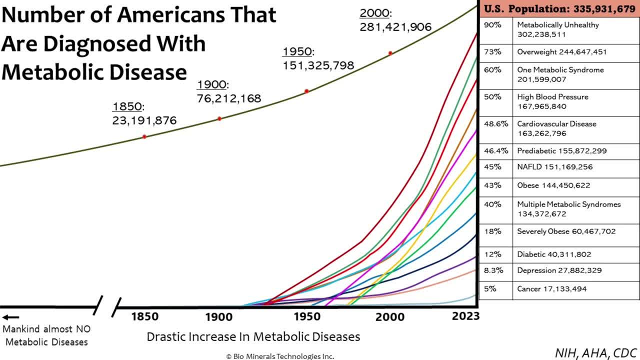 is severely obese. Over 60 million people- 40 million people in America- are diabetic. We have almost 28 million people suffering from anxiety and depression- 8.3% of our population and 5% or almost 17 million people are living. 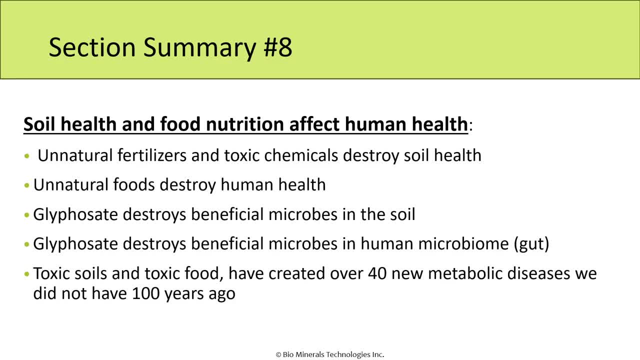 with cancer. Section 8 summary: Soil health and food nutrition affect human health. Our unnatural fertilizers and toxic chemicals destroy soil health and soil microbiology. Unnatural foods destroy human health. Glyphosate destroys beneficial microbes in the soil And it also. 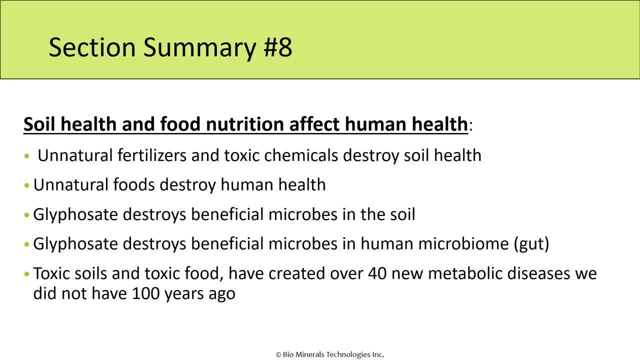 destroys beneficial microorganisms in the human microbiome, our gut. Toxic soils and toxic foods have created over 40 new metabolic diseases that we did not have 100 years ago.